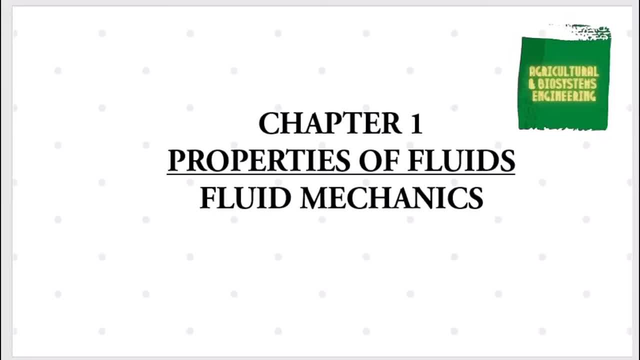 Welcome to my channel. This time I will be showing you solutions on the problems about properties of fluids under fluid mechanics. But before that, please subscribe and don't forget to click the notification bell after you watch this video. This time we will be. 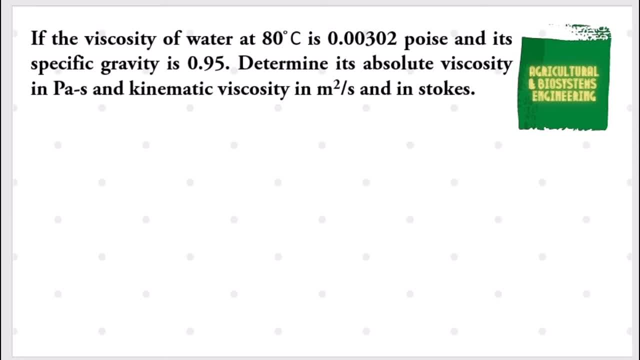 solving this problem. If the viscosity of water at 80 degrees Celsius is 0.00302 poise and its specific gravity is 0.95.. Determine its absolute viscosity in Pascal. second and kinematic viscosity in square meter per second and in stokes. The first thing we are going to identify are the 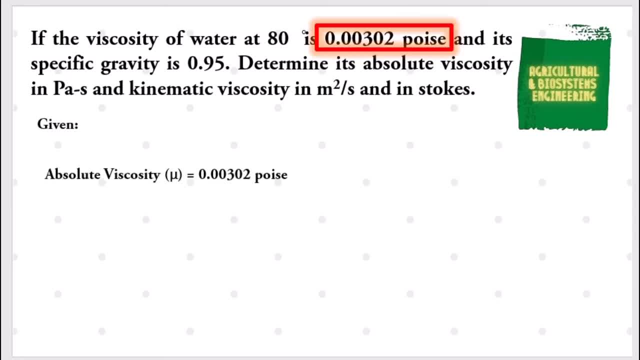 given, which are the absolute viscosity of 0.00302, poise, the specific gravity of 0.95.. And we have to add the density of water of 1000 kilogram per cubic meter. This is a constant value. It is not stated in the problem, but we will be using this later on our solution. 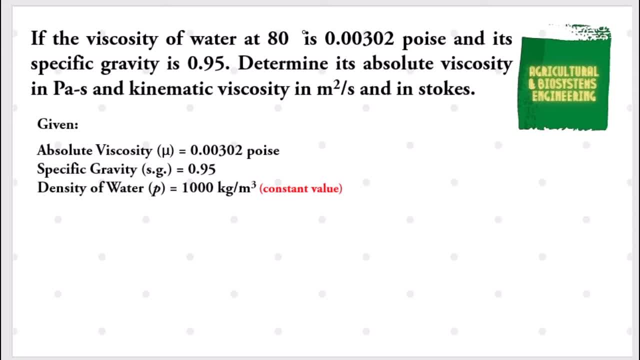 in solving the kinematic viscosity. What is required in the problem are the following: First, the absolute viscosity in the unit of Pascal seconds. Second, is our kinematic viscosity in the unit of square meter per seconds and in the unit of stokes, After determining our given. 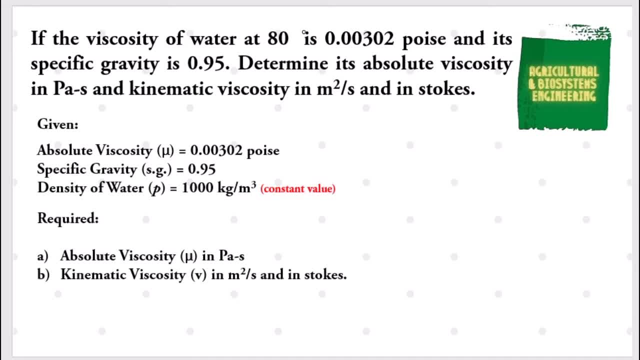 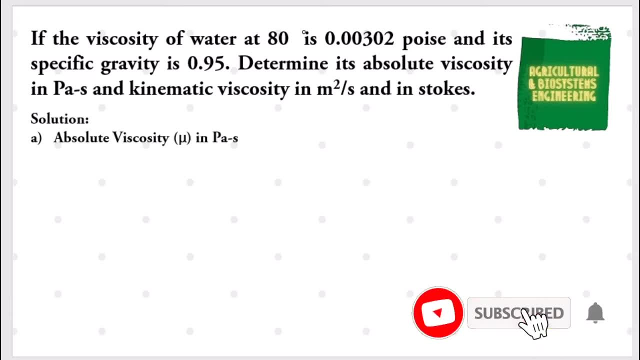 and the requirement in the problem. let us proceed now in our solution. First, that we are going to solve is for the value of our absolute viscosity in the unit of Pascal. second, To solve for that, we will simply use the conversion factor of poise to Pascal. second, 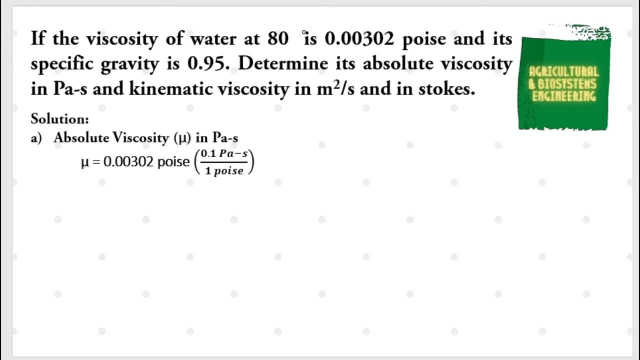 In the problem. we have a value of viscosity to be 0.00302 poise. With this value we only need to convert it with our conversion factor of 1 poise is equal to 0.1 Pascal second. we multiply and the answer is 0.000302 pascal second. that is now the value for our absolute. 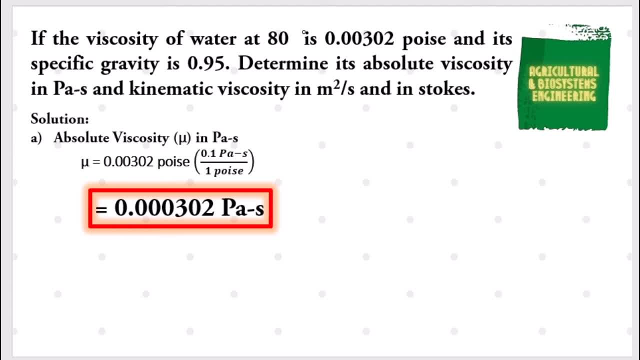 viscosity in the unit of pascal seconds. next we proceed in solving the value of our kinematic viscosity in the unit of square meters and in the unit of stokes. we begin solving with the unit of square meters per second. to solve for that we will be using the formula kinematic. 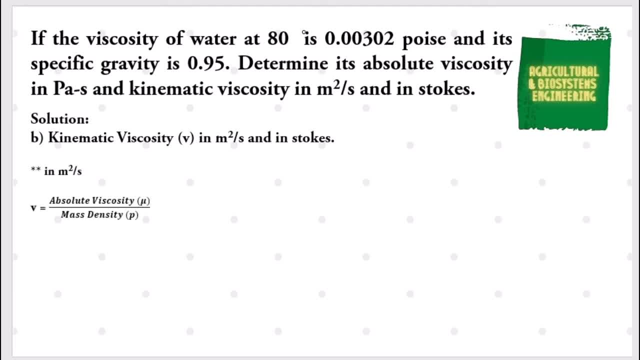 viscosity is equal to the quotient of absolute viscosity all over the mass density. however, we still don't know the value for our mass density, so we have to solve for its value using the formula: mass density is equal to the product of the density of water multiplied to the specific 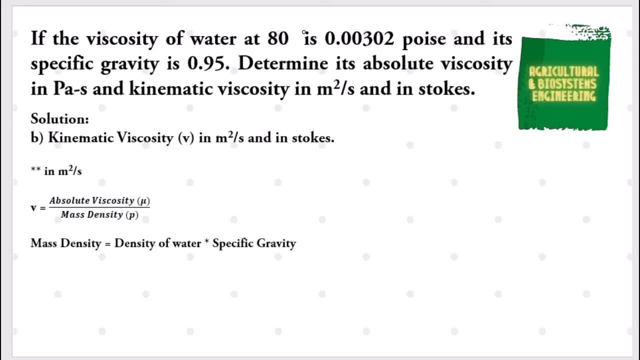 gravity. we already identified a while ago that the density of water has a constant value of 1000 kilogram per cubic meter. also, the specific gravity of the mass density is equal to the product of the density of water multiplied to 0.95. as stated in the problem, we simply substitute the values and we have 1000 kilogram per cubic. 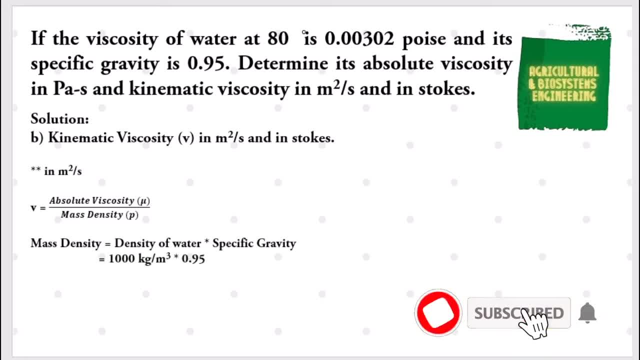 meter multiplied to 0.95, we now have a value of our mass density of 950 kilogram per cubic meter. now that we identified the value of our mass density, we go back in the formula to solve for our kinematic viscosity in square meter per second, the value for our absolute viscosity. 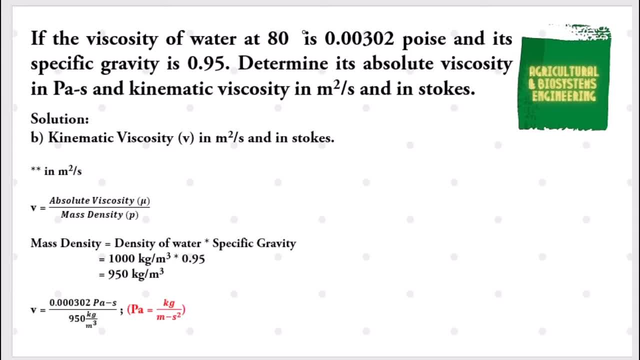 is the value we solved a while ago. so we simply use direct substitution and we have: kinematic viscosity is equal to 0.000302 pascal second, all over the mass density of 950 kilogram per cubic meter. before we get the quotient, we know that pascal unit is also the same as kilogram. 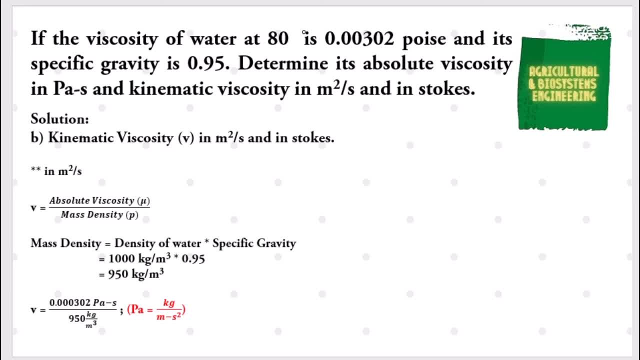 per meter by square. second. with these we substitute it to the unit of pascal and we have: v is equal to 0.000302 kilogram per meter by square. second by second, all over 950 kilogram per cubic meter. if you noticed in the numerator, we can cancel out the second unit. now we know that. 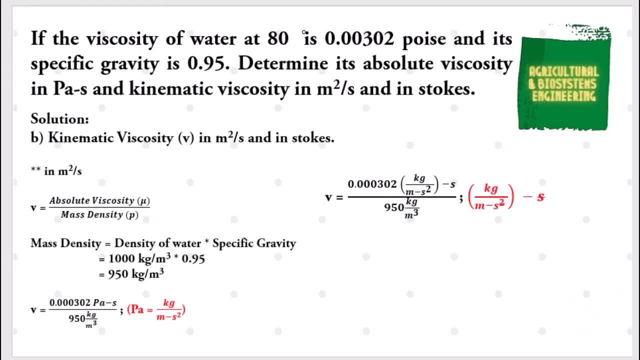 0.000302 kilogram per meter by second. all over 950 kilogram per cubic meter is the same as multiplying 0.000302 kilogram per second. all over 950 kilogram per cubic meter is the same as multiplying 0.000302 kilogram per meter by second to the reciprocal of the denominator. 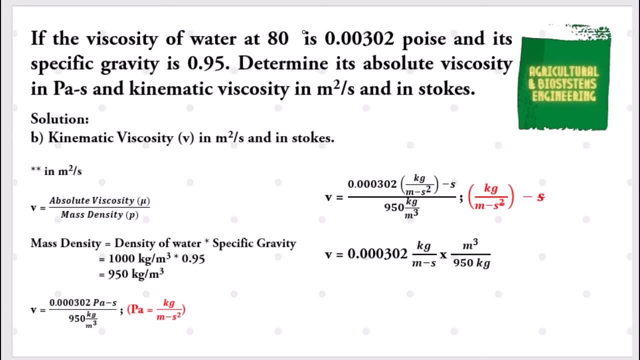 which is now cubic meter all over 950 kilogram. we simply get the product and we cancel out the kilogram unit and the one meter unit to leave is square meter. now we simply solve and the answer now is 3.18 times 10, raised to negative, 7 square meter per second. that is now the value of our